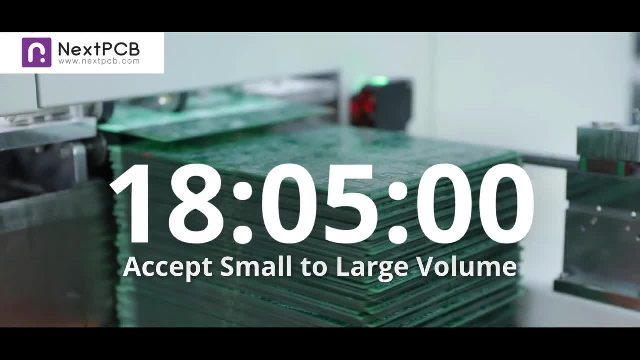 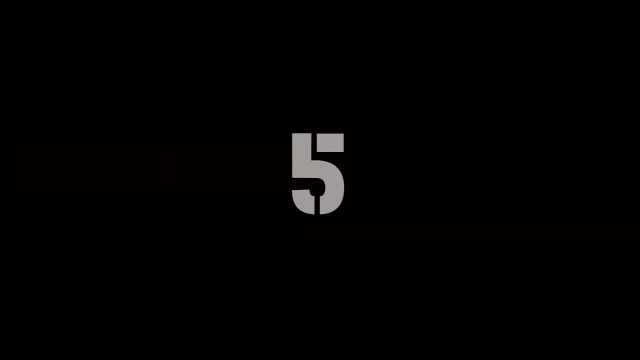 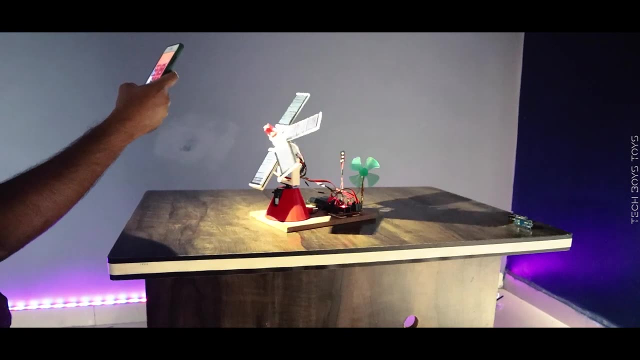 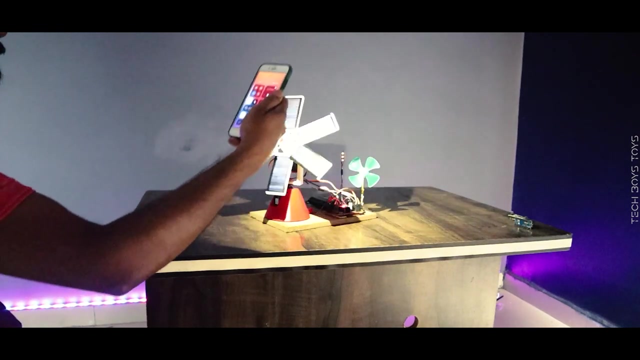 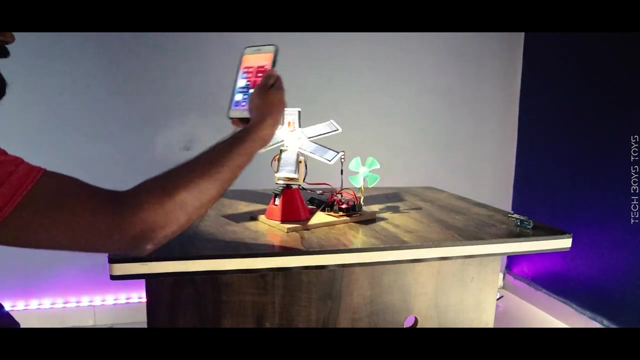 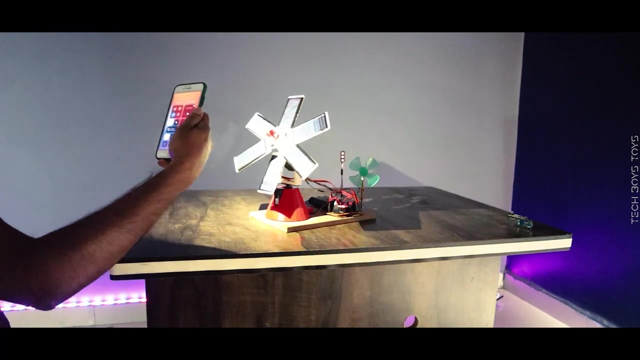 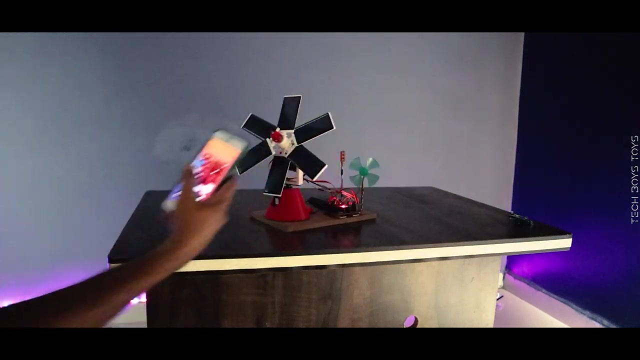 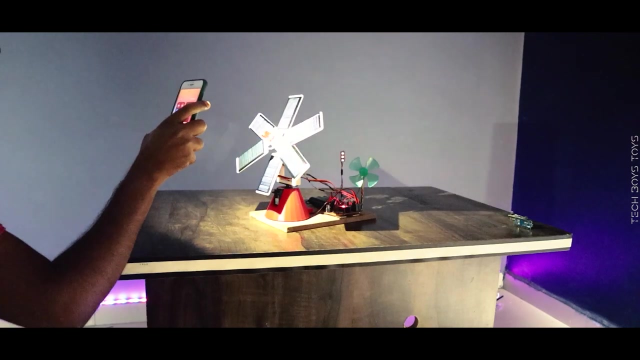 Next, PCB is your complete solution for printing circuit board. Please check the description for more information. Number 5, Number 6, Number 7, Number 8, Number 9, Number 11, Number 12, Number 14, Number 15, Number 16, Number 17. 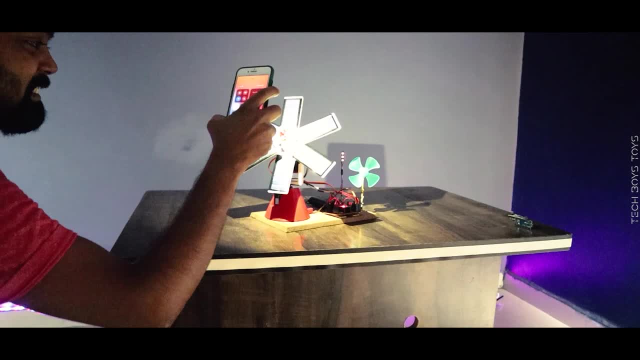 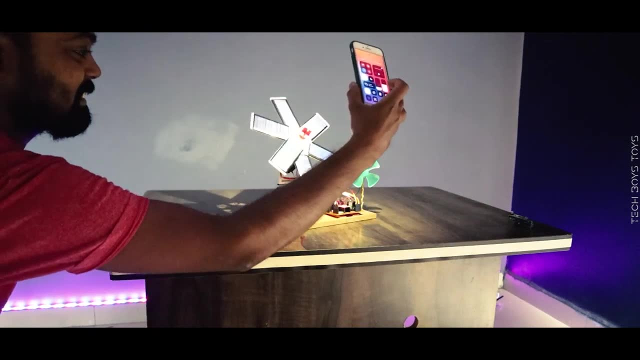 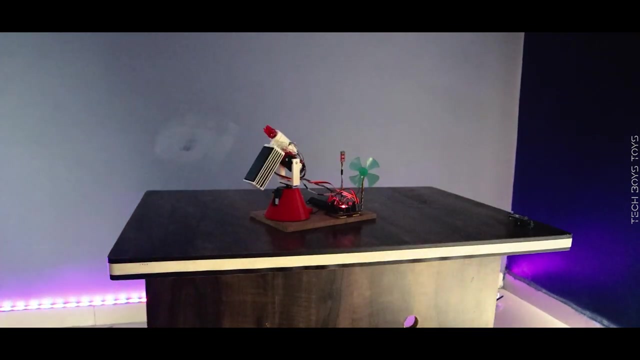 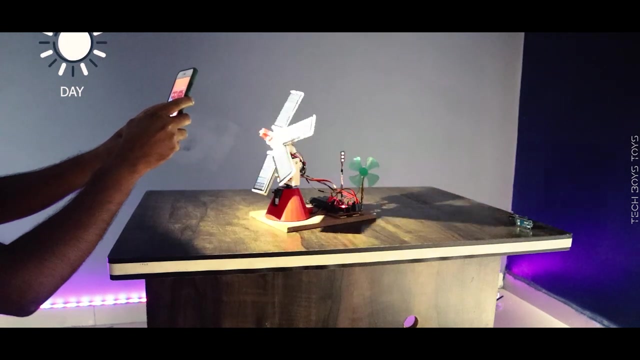 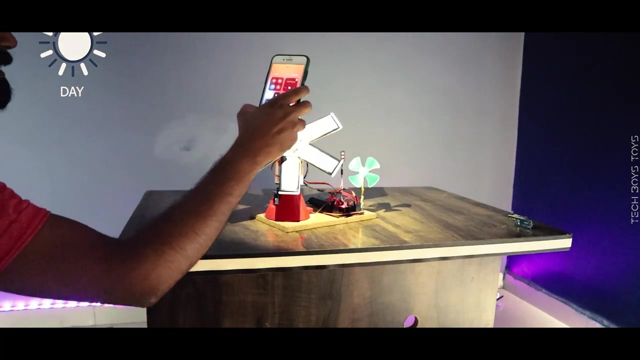 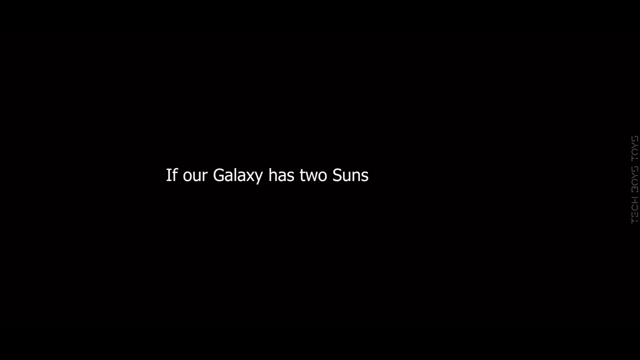 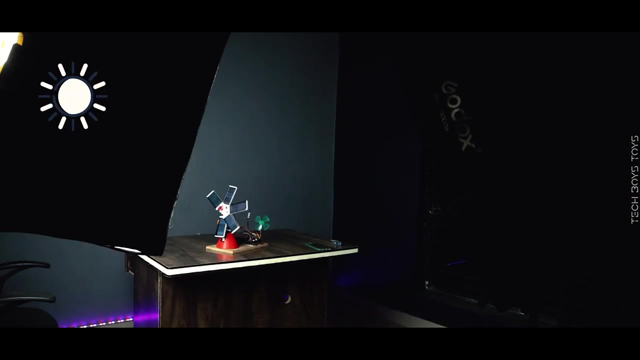 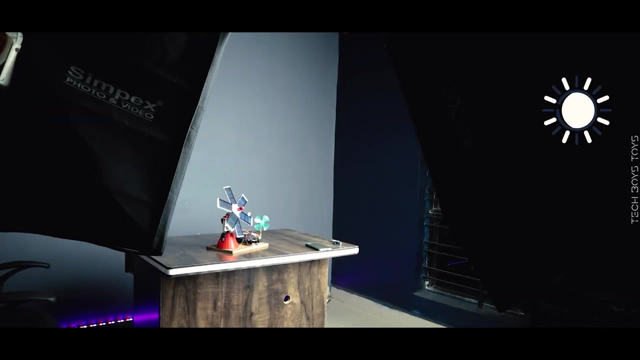 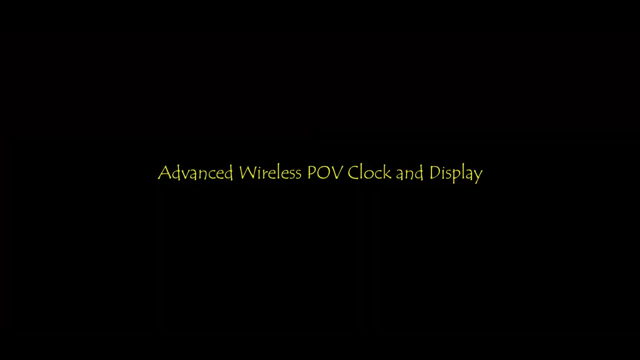 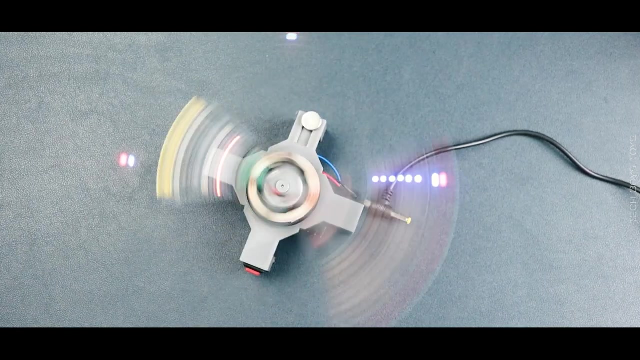 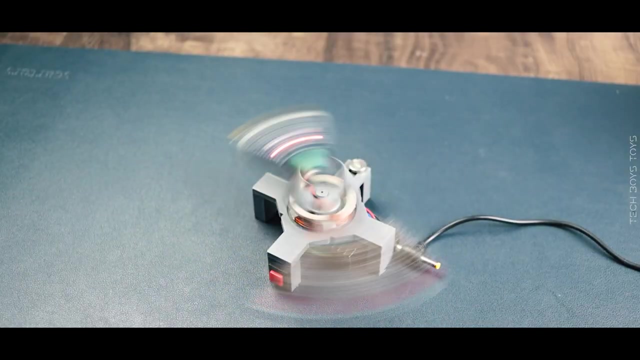 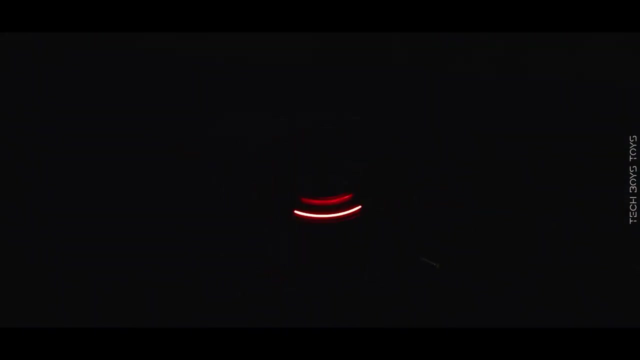 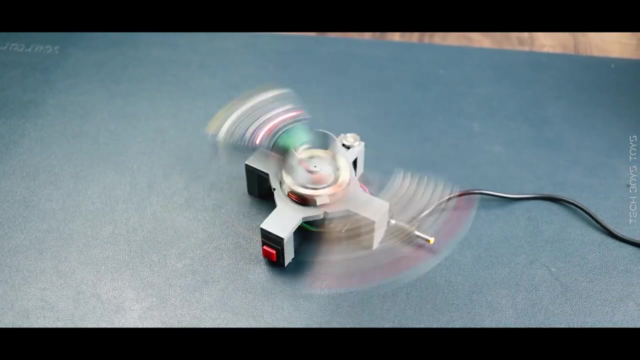 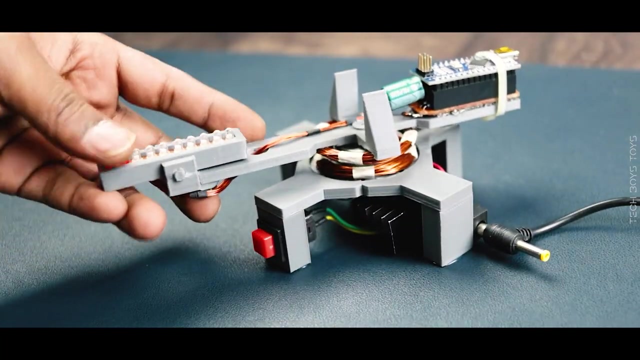 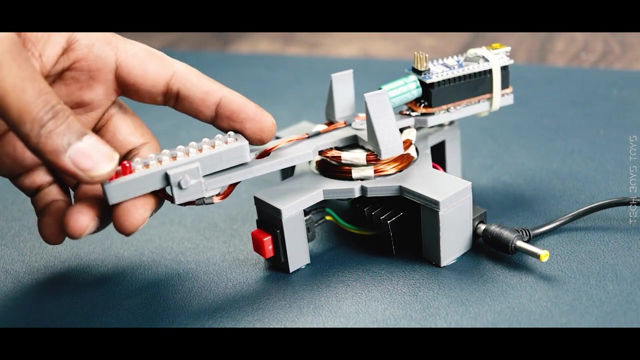 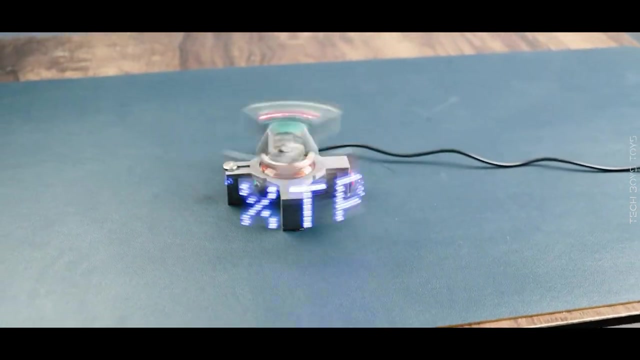 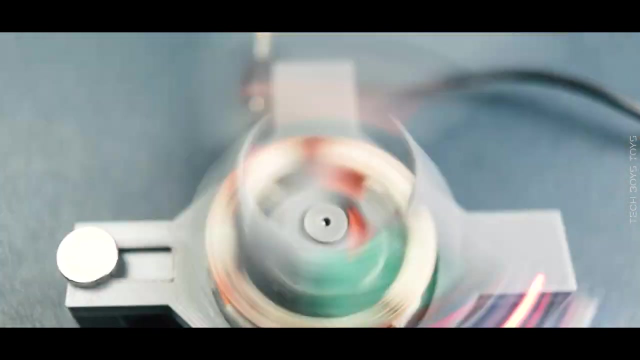 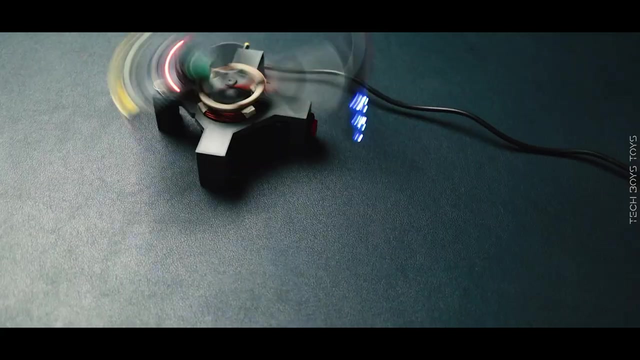 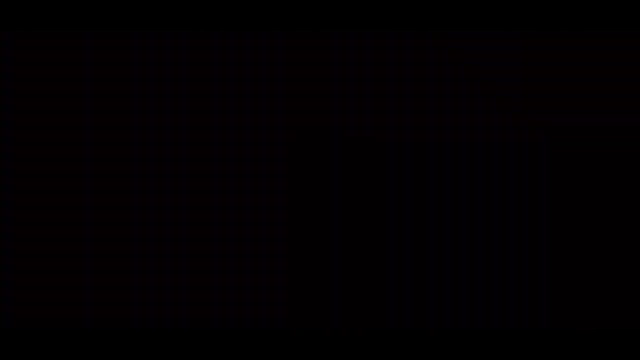 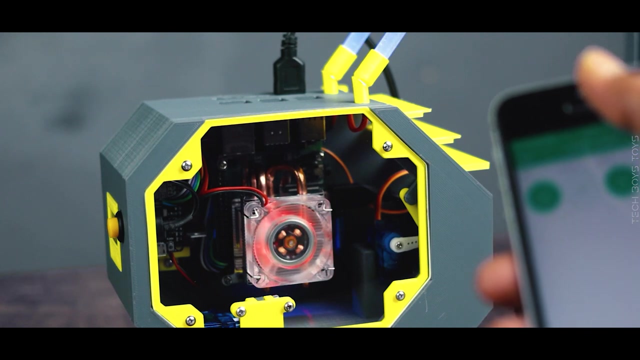 Number 18, Number 19, Number 20, Number 31, Thank you. Number 4, Number 5, Number 6, Number 7, Number 8, Number 9, Number 10, Number 11, Number 12, Number 13, Number 14, Number 15. 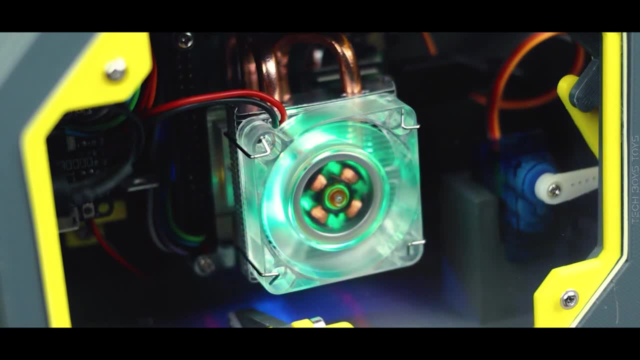 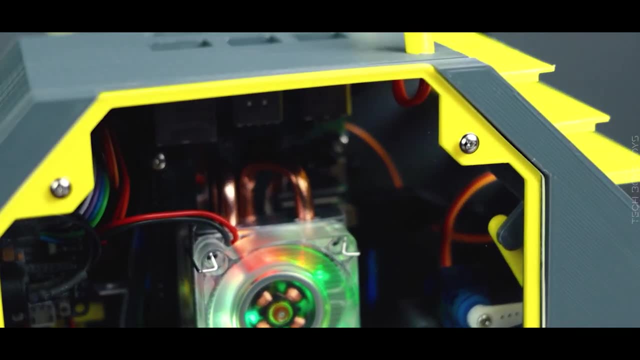 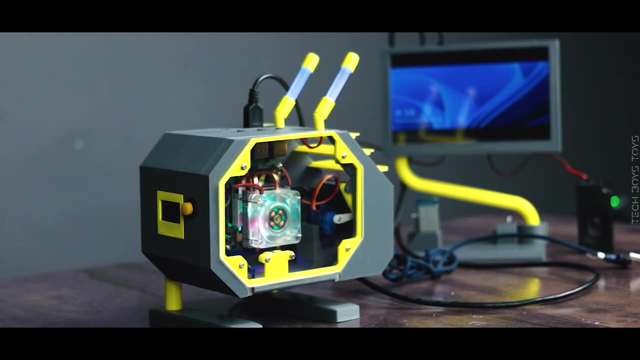 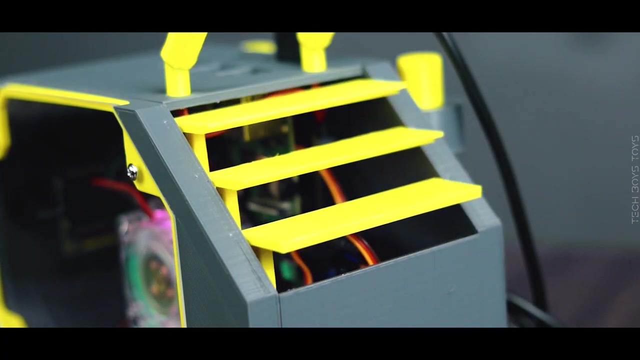 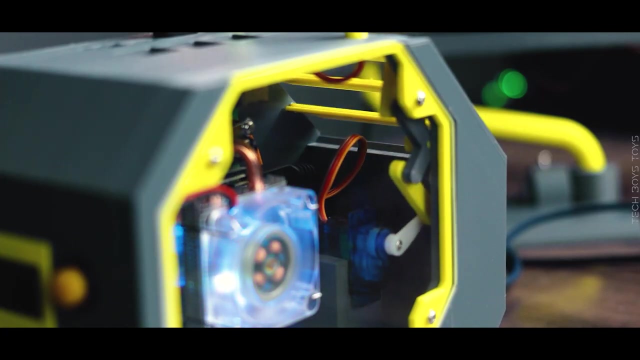 Number 16, Number 17, Number 18, Number 19, Number 20, Number 21, Number 22, Number 23, Number 24, Number 27, Number 28, Number 29, Number 30, Number 31, Number 32, Number 33, Number 34. Number 35, Number 36, Number 37, Number 38, Number 39, Number 40, Number 41, Number 42, Number 45, Number 46, Number 48, Number 49, Number 51, Number 52, Number 53, Number 54, Number 56. 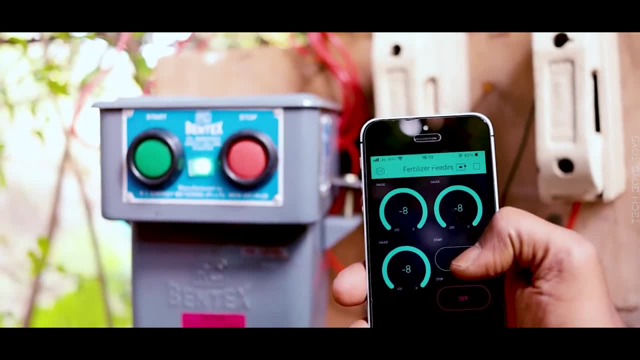 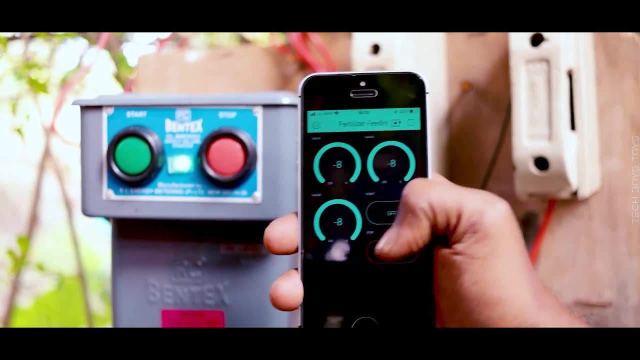 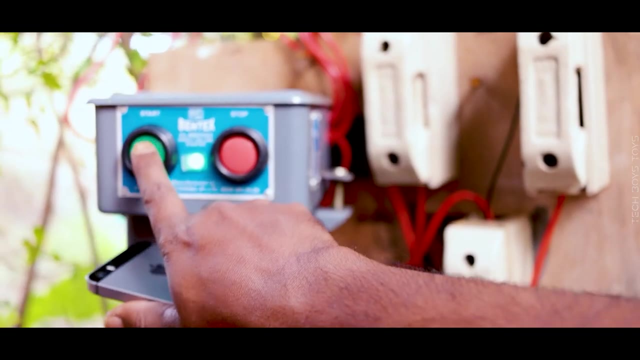 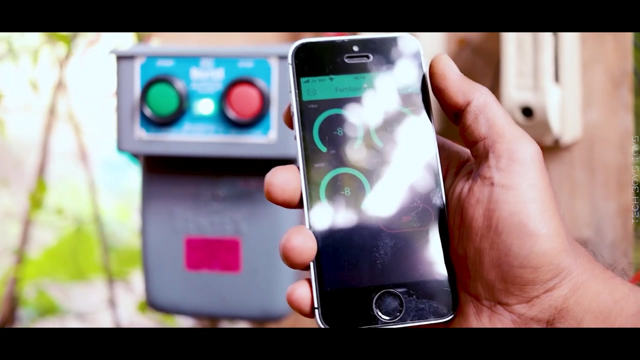 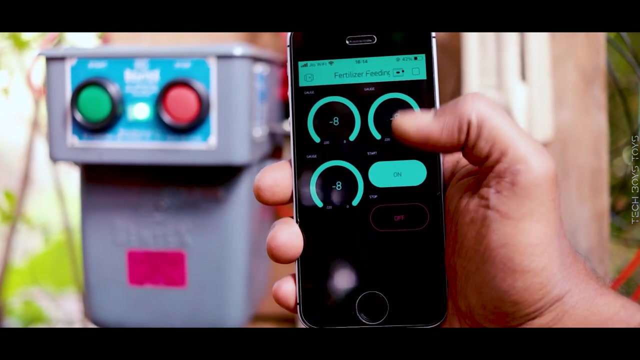 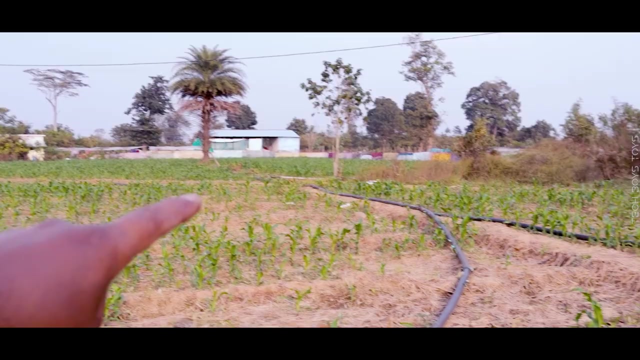 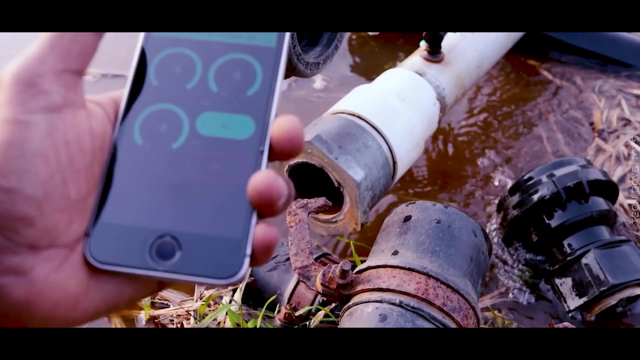 Number 57: 1946. okay. okay, it's turn on right now and it's off. okay, we can do this manually also. it's turn on, turn off, okay, and also we can do this from this. it's turn on and right now it's turn off. there is our pump, there is the pipeline.